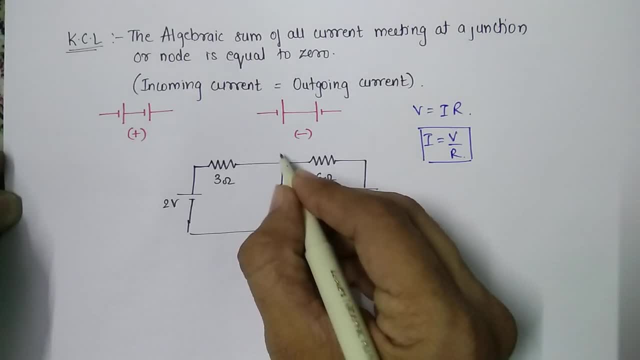 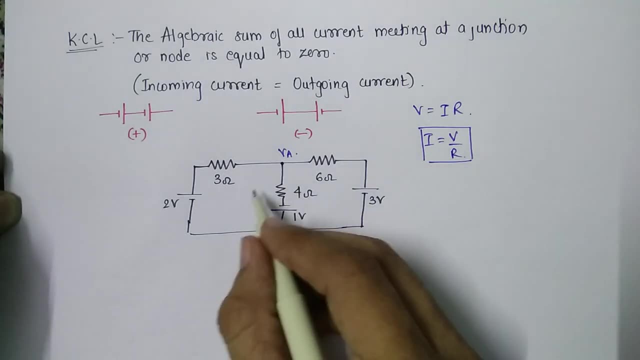 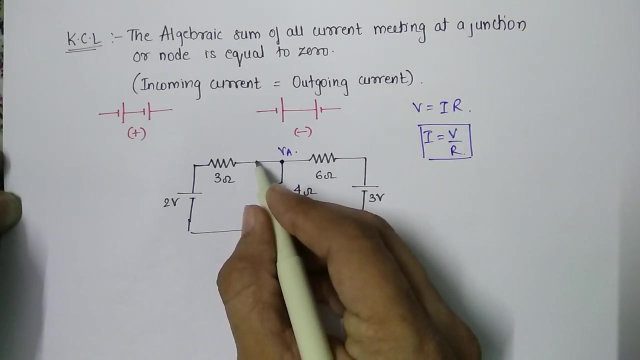 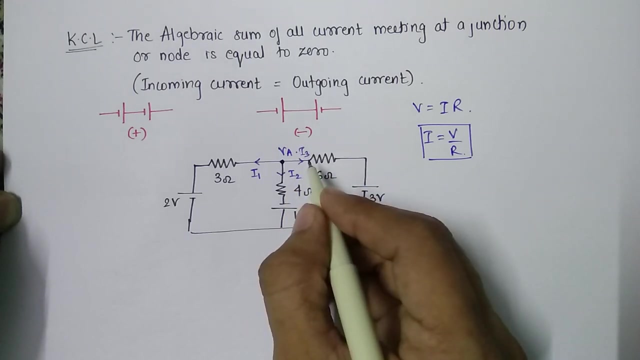 be using this to solve this circuit and find out the voltage at this node. I'll assume it had to be VA, So this thing is also sometime called as nodal analysis. Now, guys, how to relate this nodal analysis. See, I'll be applying KCL at this node. If node current is not mentioned, I'll always assume away I1, I2 and I3.. These are the node, This is the node voltage, And if the current is not given, you'll always assume away I1, I2 and I3. 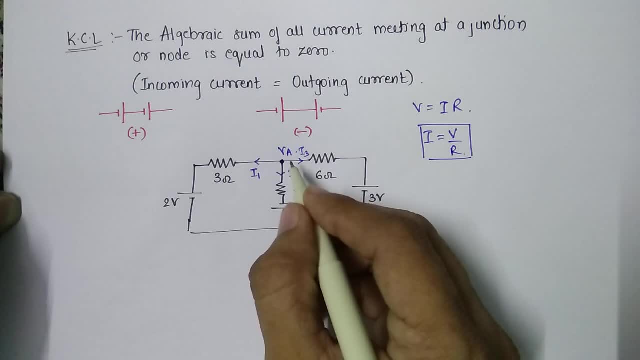 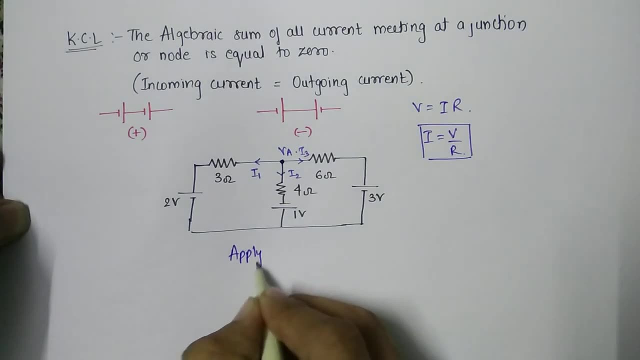 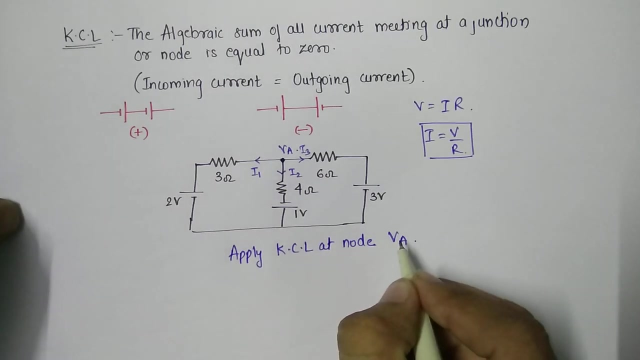 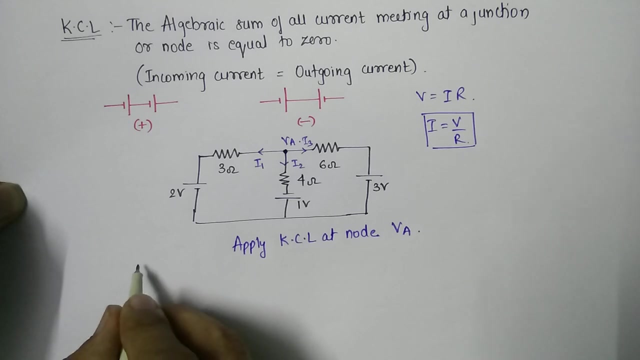 away from the junction. you can assume incoming also, but I'll assume always away from the junction. Now I'll apply KCL at this node, So applying KCL at node VA. Now, if you apply KCL at node VA, what will happen is see, I'll write first a very small relation like I1 plus I2 plus I3.. 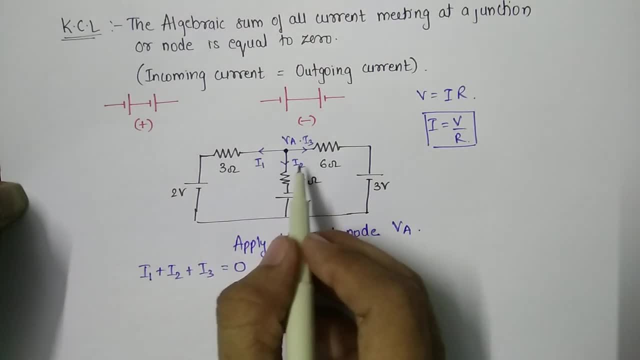 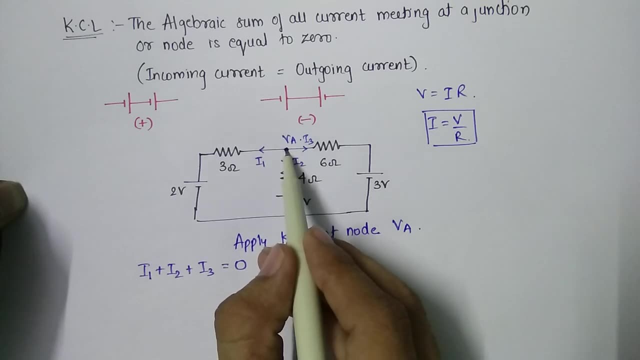 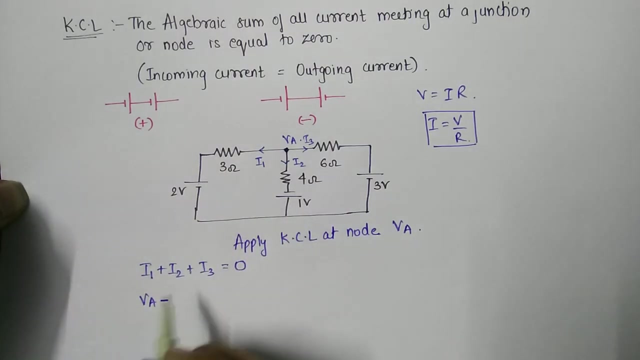 is equal to zero, since all the current are moving away from the junction, There is no incoming current. Now, guys, I equal to V by R, So I1 will be this is. I'm considering this to be at higher potential, So I'll write VA minus this voltage, Since this is also at higher potential, this is also at higher potential When there is two terminal at higher potential will subtract the VA minus two upon three. Next will be: 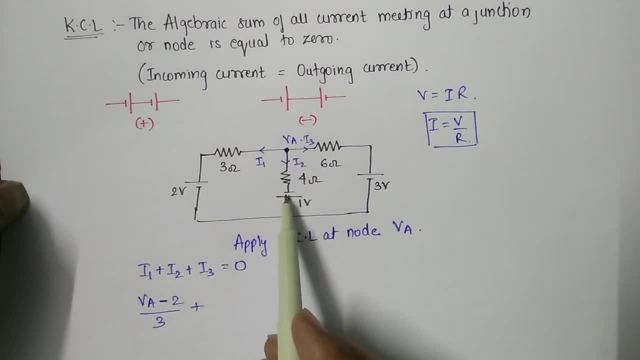 Next voltage will be VA. See this, we have negative potential. So if higher potential and negative potential will add, So I'll write VA plus one upon four. And finally, the third equation: VA minus three. Since this is also at higher potential, this is also at higher potential. VA minus three upon six is equal to zero. Now you have one equation. 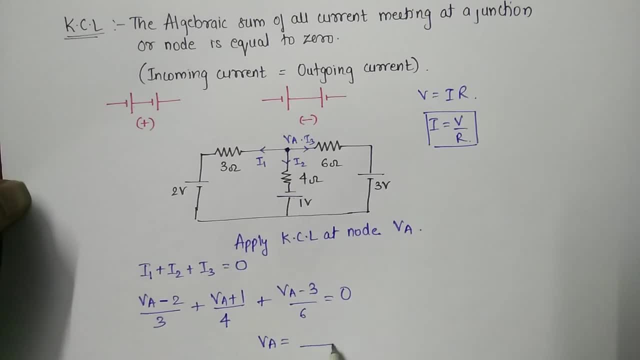 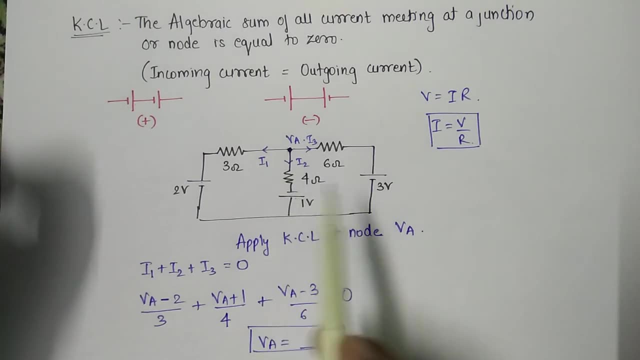 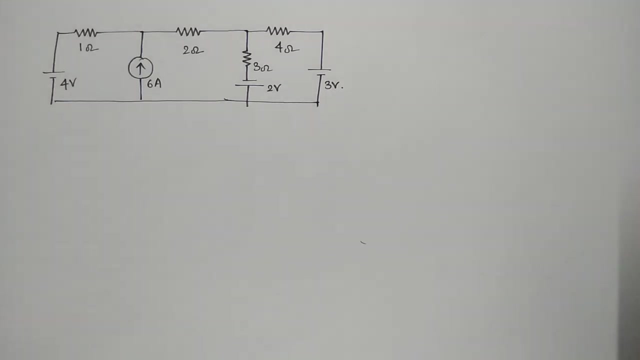 And one unknown. So we can directly calculate the value of VA, either using calculator or simplifying it. So this is one way, or one node now assume, or I'll solve using two node. Okay, so let's take another problem to solve to. Okay, now let's take this example to solve. 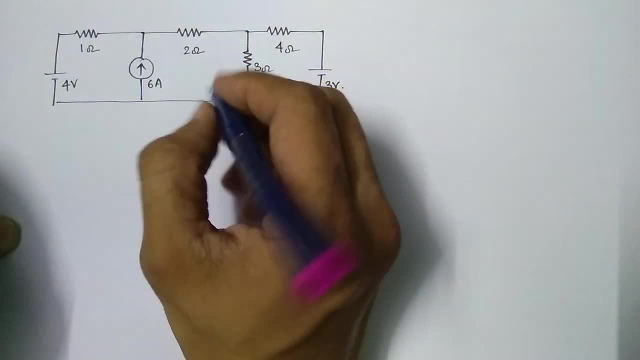 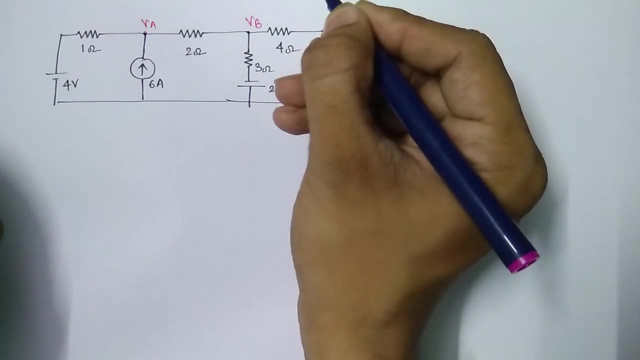 model analysis or how to apply KCL. So I'll assume two nodes over here. One, I'll name it where it is actually given 200 hits Here, where it is actually given200 hits, VA. another, I'll name it as VB. please remember that concept. if there is a 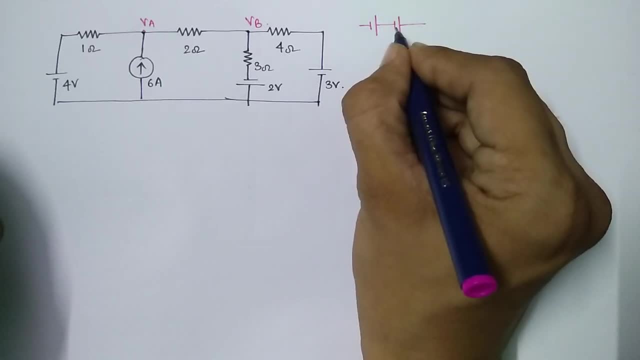 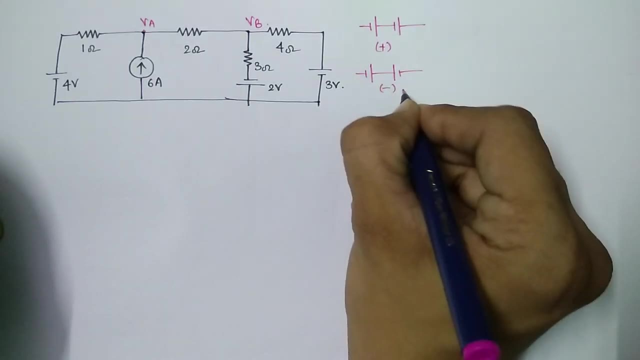 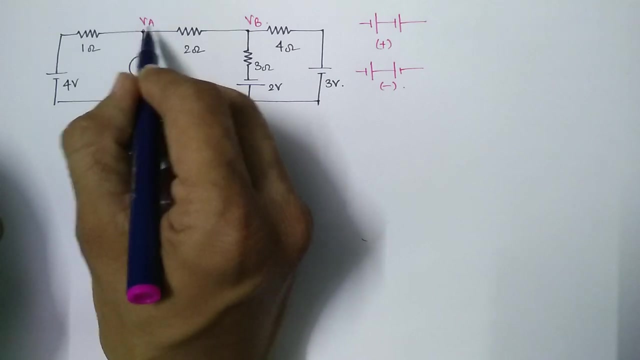 positive terminal and a negative terminal connected to each other of a battery will add the voltages. if positive is connected back to positive, will subtract the voltages. okay, now apply KCL on VA. first see whenever you considered see, I can also consider VA, VB, VC, VD. it depends on you how much node. 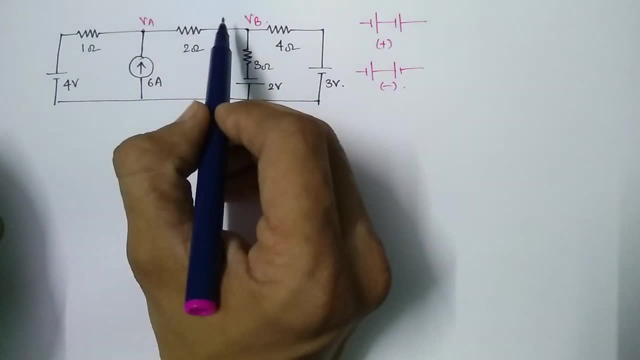 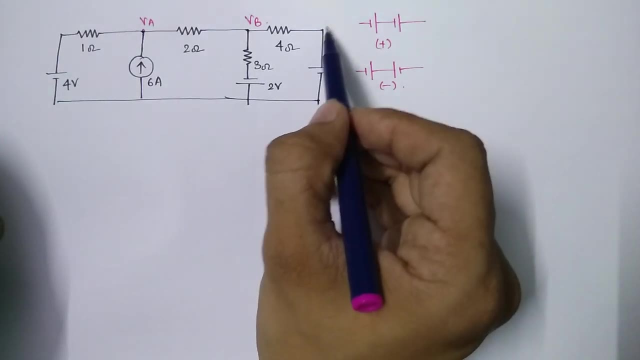 you can consider, but when examiners give you two nodes, you have to use two nodes. but if I assume VA to be this node, guys, you can directly write VA as 4 volt. if you consider VDS 3 volt, you can directly write VDS 3 volt. okay, so if you? 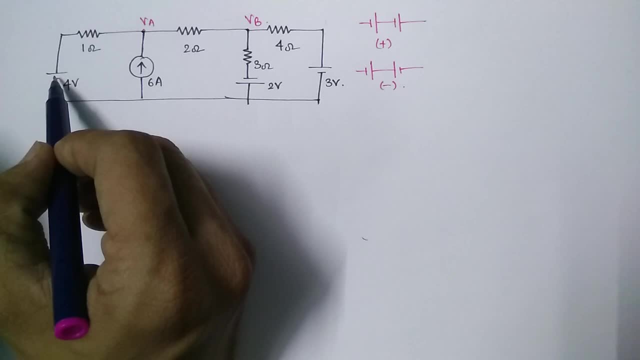 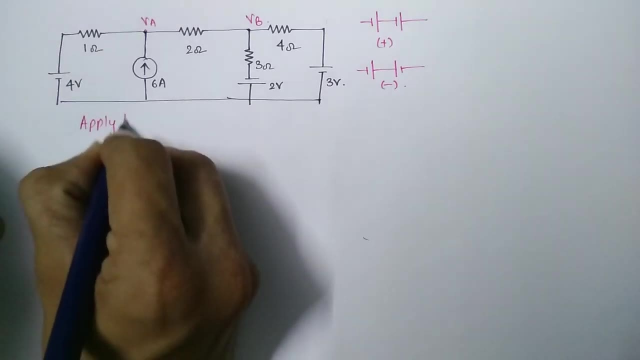 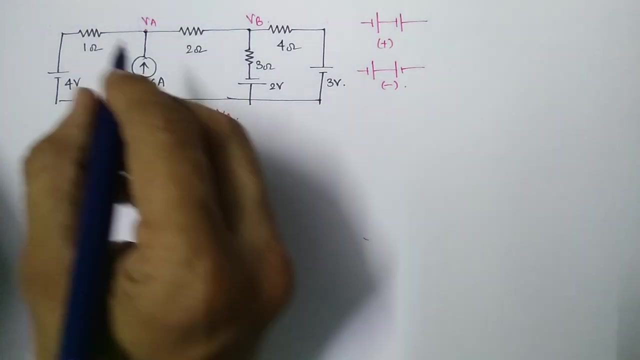 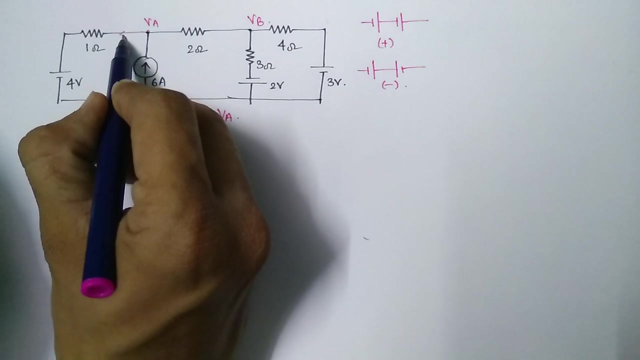 consider node next to voltage, the node will have the same voltage. it's a basic fundamental. now I'll apply KCL. I'll apply KCL at node VB, VA. so when I apply KCL at node VA, so guys see how many are income incoming and how many are outgoing current. if current is not mentioned, I'll assume away. 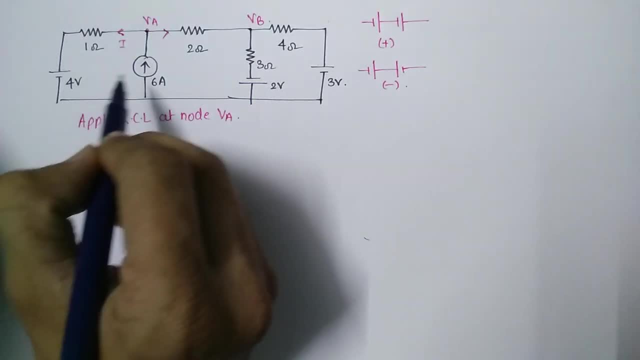 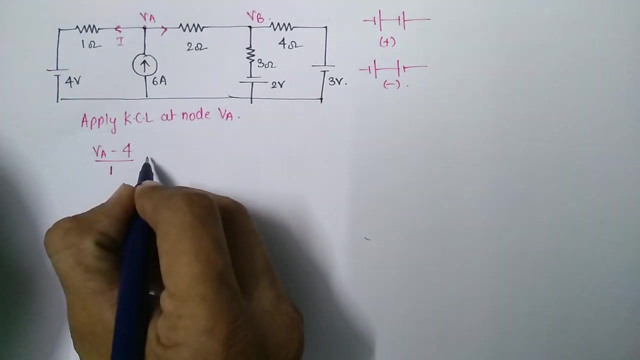 if current is not mentioned, I'll assume away. but here current is mentioned, so we'll consider to be at incoming current and this two should be at outgoing current. so now, VA minus 4 upon 1 next will be: see, this is incoming. will write on that dead side of equation, so now I'll write. 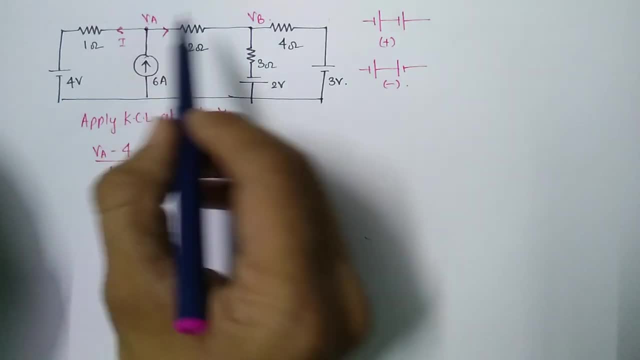 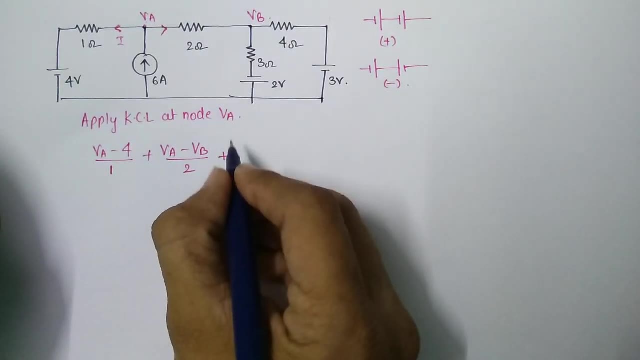 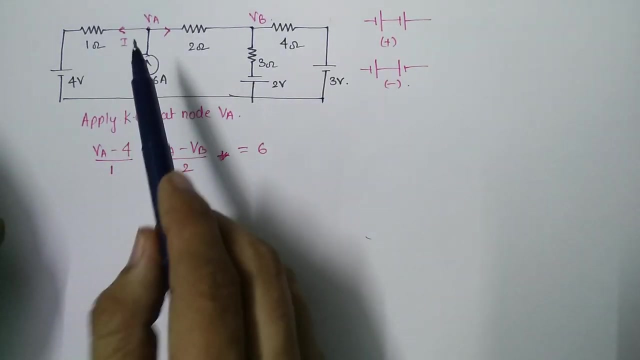 VA. this is higher potential. this is also higher potential. so VA minus VB upon 2. and finally, we don't have any another incoming current, outgoing current. we have incoming current, so you won't write anything over here, will write equal to. we have one incoming current, will write 6 ampere. so this is first equation in which 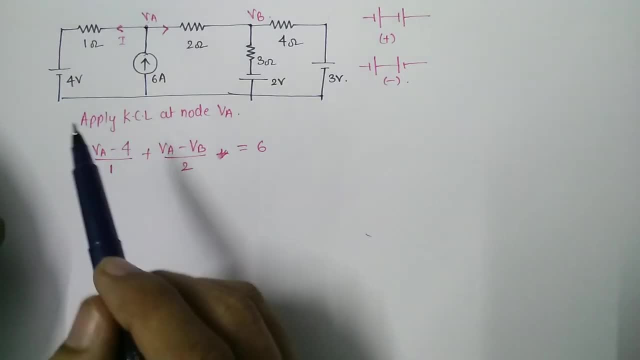 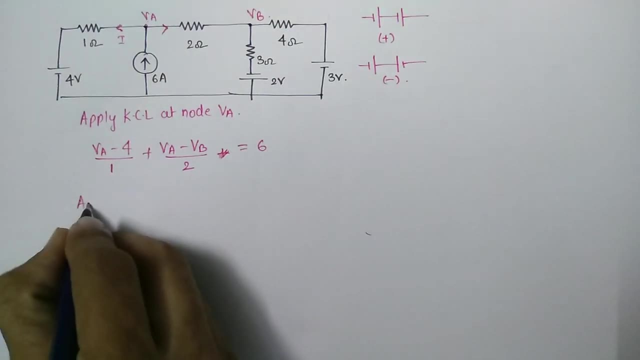 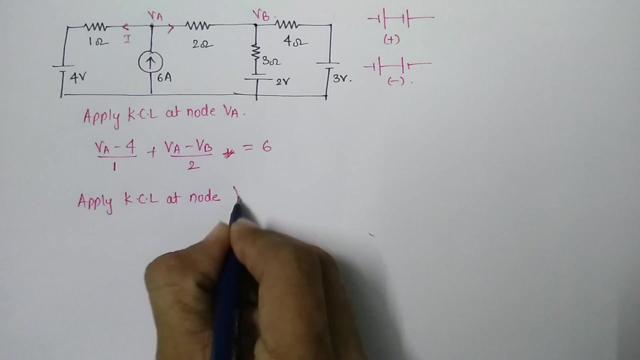 you have written VA and VB. you simplify it. you'll get a equation in terms of VA and VB. now let's take another node VB. I'll apply KCL at node VB. now what will happen if I apply KCL at node VB? guys, if the direction is, 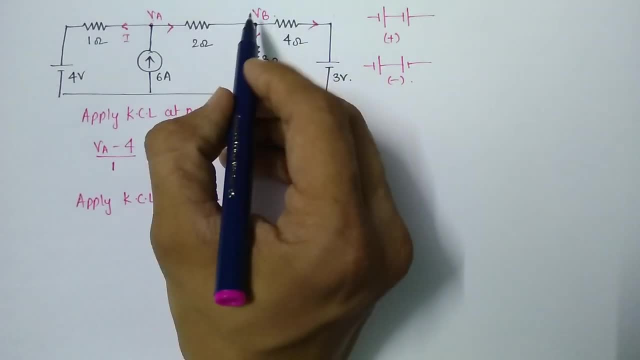 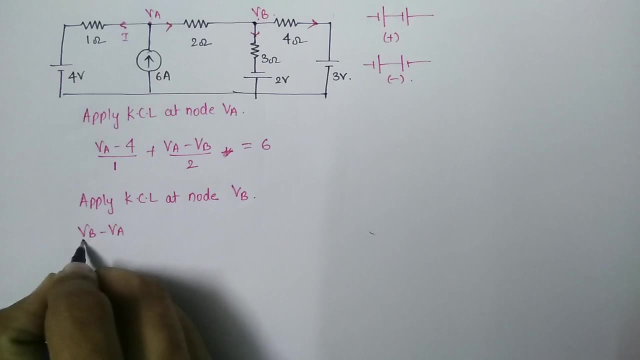 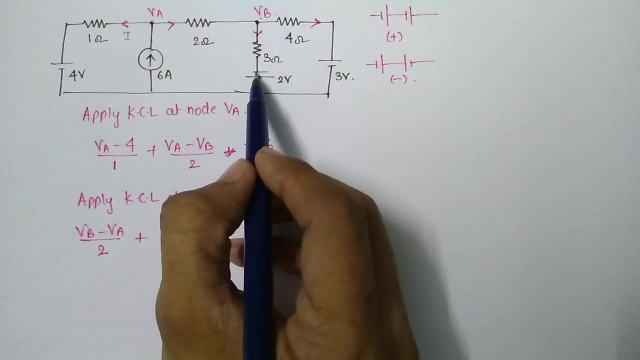 not given, I'll assume away. away now. see, this is at higher potential. this is also word higher potential. so VB minus VA upon 2. next will be this current VB, since it is higher potential, this is lower potential, and we have higher and lower, we should add. so VB plus 2. 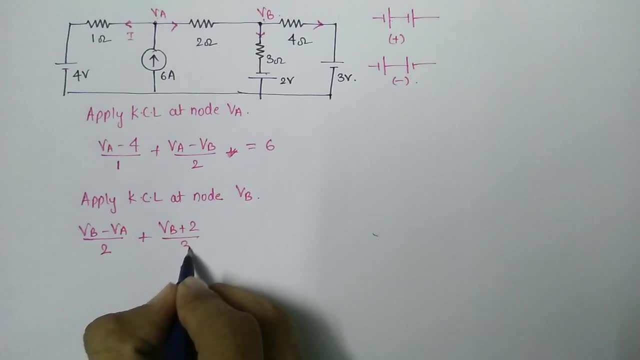 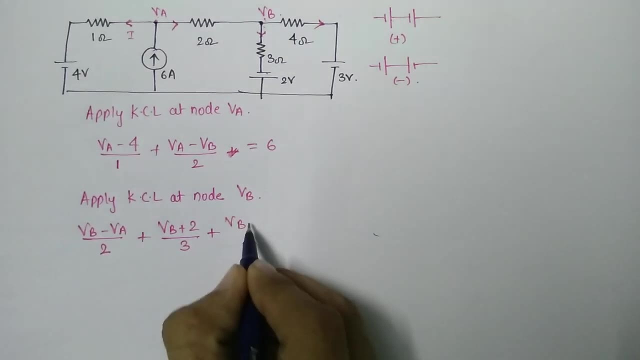 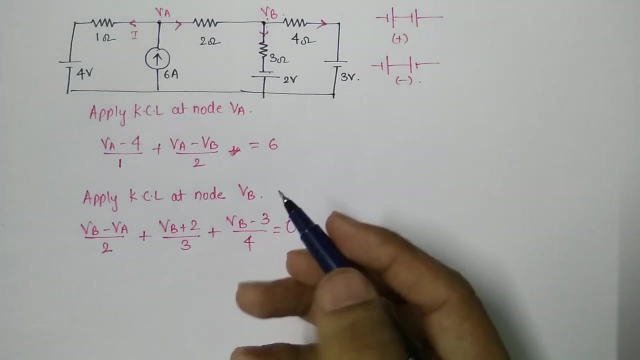 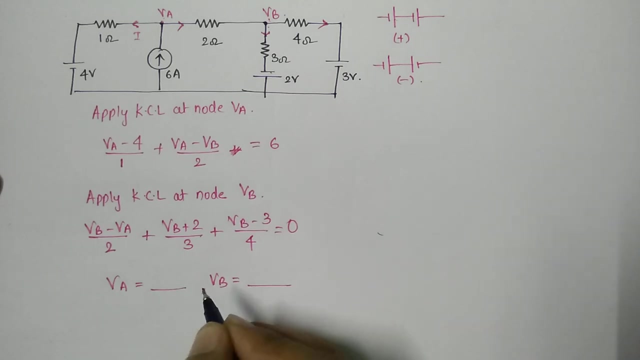 I'll write VB plus 2 upon 3 and finally I'll write VB minus 3 upon 4, minus 3 upon 4, equal to 0. now you have two equation and two unknown. you can easily get the value of VA and VB, either use simultaneous equation or use calculator method. so hope you. 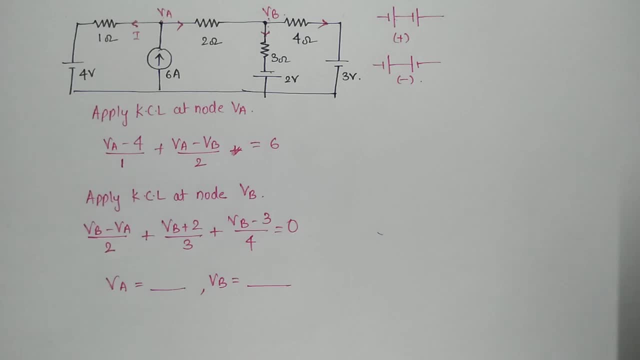 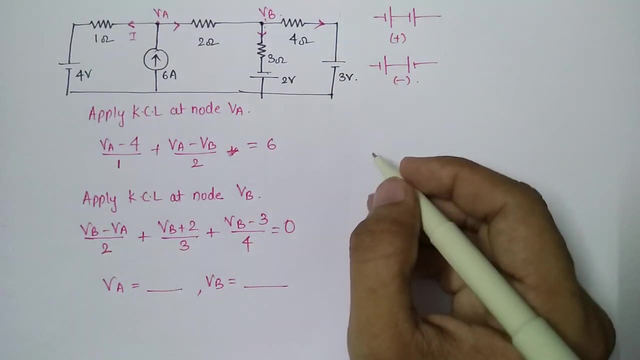 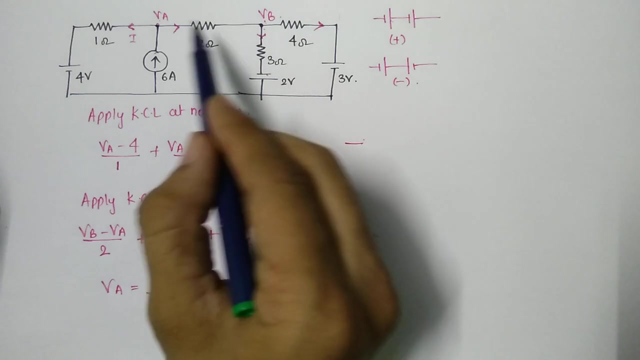 understand this video, guys. there are another small concept and which can be, which can be very important while designing some equation or circuit. see if you, if there is, if there is, see this is: there are two nodes, VA and VB. I have not taught you how, if there is any voltage between two nodes, suppose there is a voltage between two. 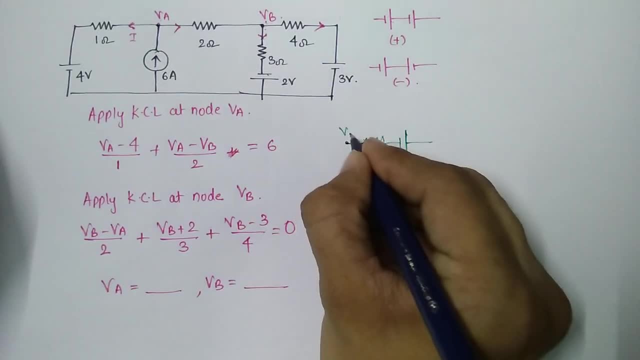 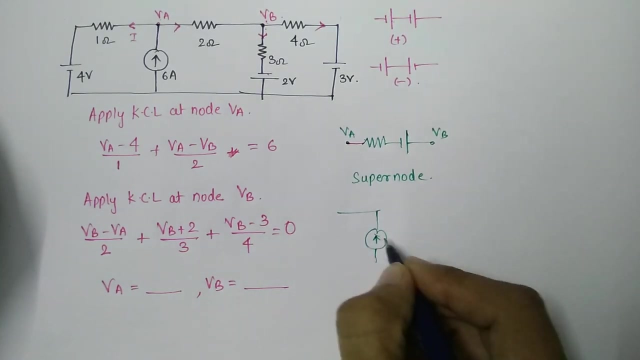 nodes. suppose there is a node voltage- VA and VB- and there is a voltage between two nodes. how to solve this? such problems comes under super node. ok, and if there is a current source like this inside any two loop, how to solve it? using KVL? that concept is known as super mesh. so how to solve this? 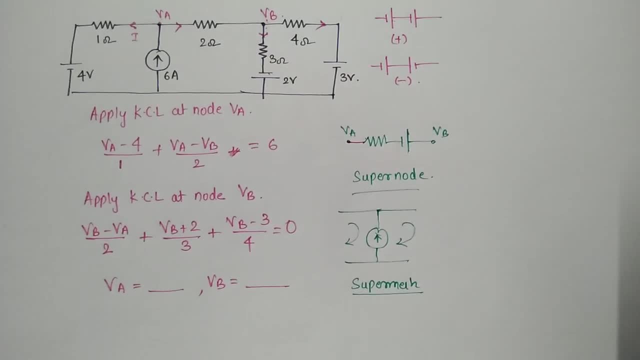 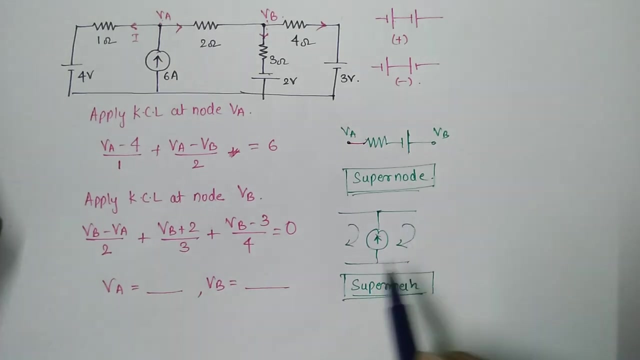 two. I'll teach you in the next lecture. so guys hope you understand what what super node says and what super mesh say. if there is any extra voltage between two nodes, that problem I will treat it as super node. if there is any extra current source like this inside any two loops, that problem is known as super.